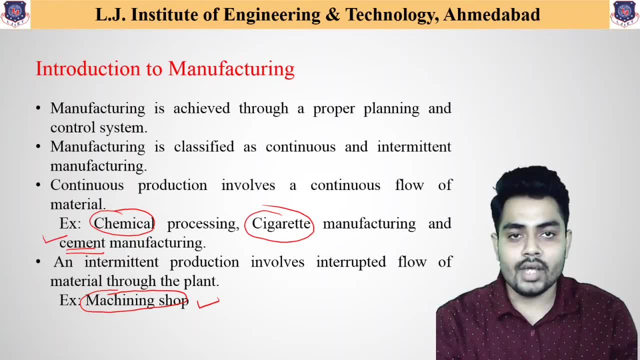 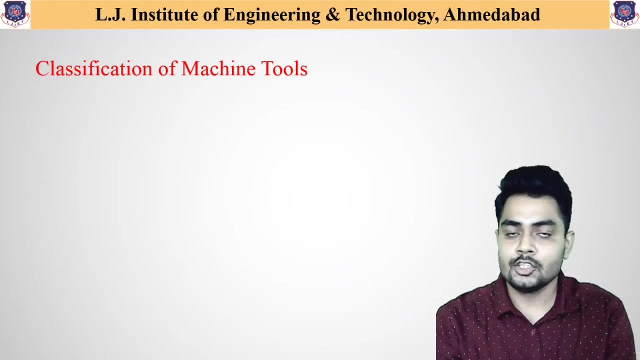 operations are performed as per the requirement, But whenever the component manufacturing is complete, all that machineries remain ideal. So machining soap is one of the example of intermittent manufacturing system. So now let us understand classification of the machine tools. So what is the first of all meaning of machine tools? So, any of the time as we 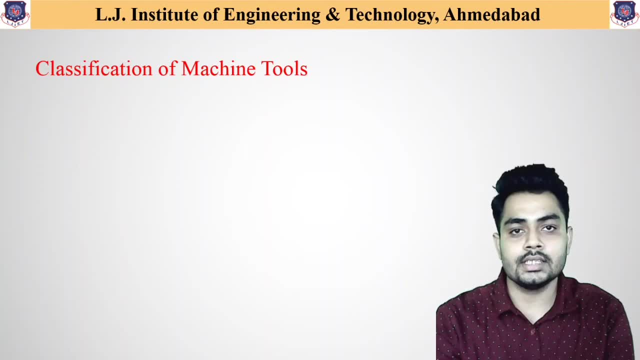 have listed: lathe machine, milling machine, saper machine- all these machineries perform a particular operation on the work piece or component. So these all machineries are nothing but the machine tools. that means the tools which are used for manufacturing or for any. 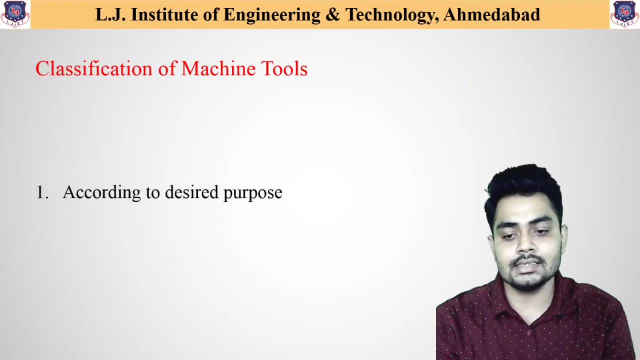 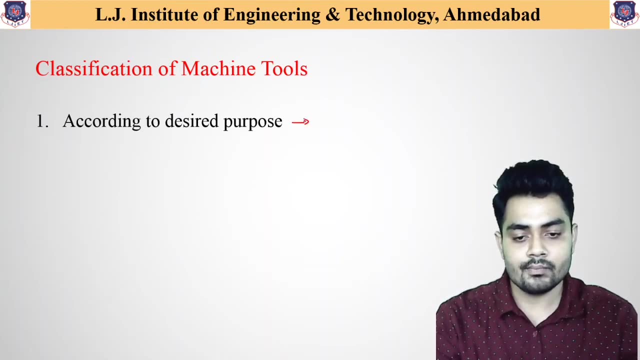 finishing or cutting purposes. So first one, that is, the according to the desired purpose. So based on that we can define it as: first one is single purpose. Second one is single purpose machine tools. Similarly it can be again defined as multi purpose machine tools. 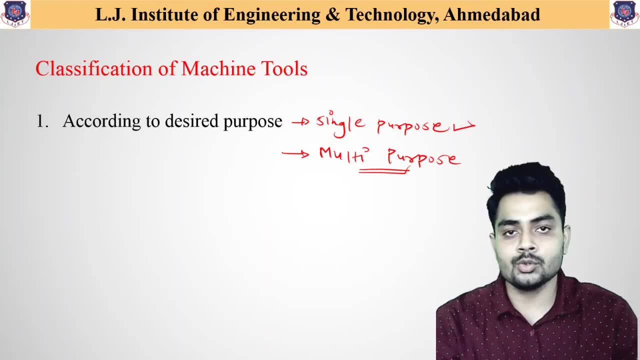 That means in the case of single purpose machine tool. if we say if any of the particular machine tool is useful for any specific one application, at that time it is called as the single purpose machine tool. And if machinery is useful for more than one operation, at that time it is called as the. 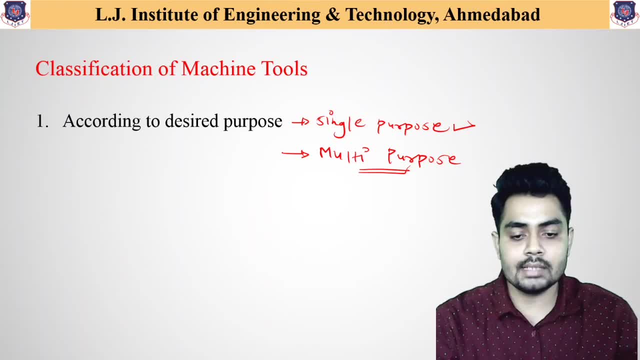 multi purpose machine tool. So if we take example of lathe machine, So we know that in the case of lathe machine different operations are performed, such as turning it may be, a threading may be facing. So all this type of different operations are performed. 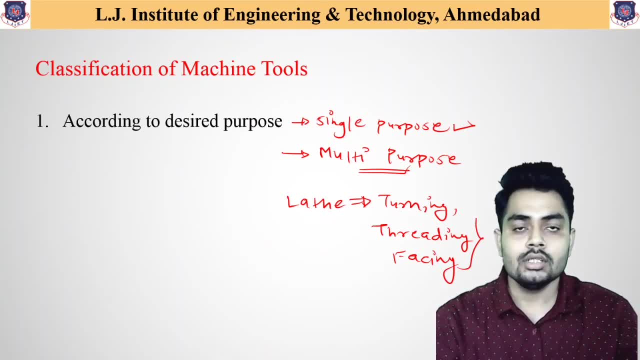 operations can be performed very easily on this lathe machine. that's why this lathe machine is called as the multi-purpose machine tool. so this is the main variation in based on the desired purpose. it may be a single purpose machine tool or it may be a multi-purpose machine tool. now let us 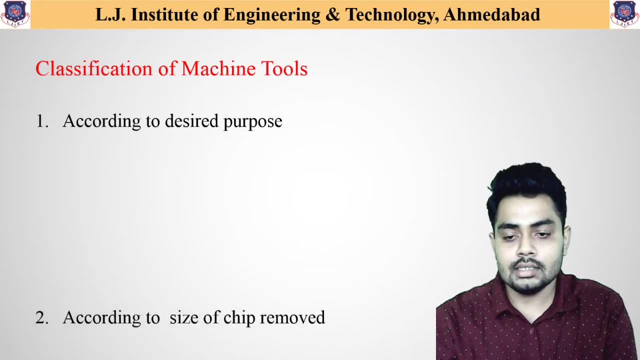 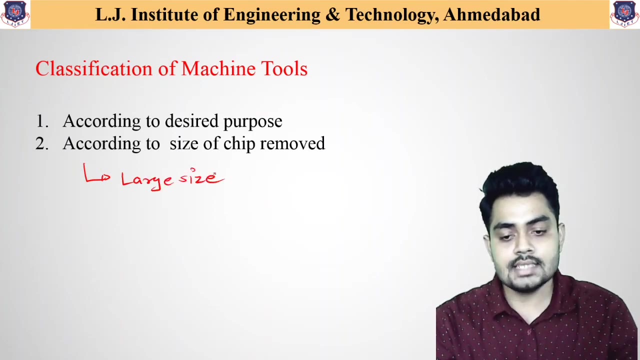 have a look at another classification, that is, the according to the size of chip removed. so, based on that, there are two variation: first one that is the large size tip removed and the second one that is the smaller size tips removed. so, based on these, if in any component the chips removed are comparatively 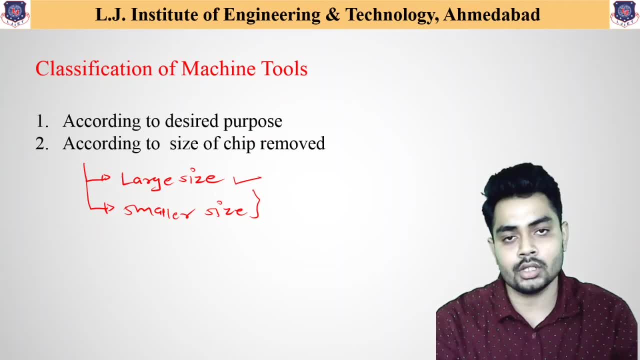 larger, then it is called as the large size tip removed component. or if the chips removed is very smaller, at that time it is called as the smaller size tip removed machine tool. so, as we have introduced different types of machine tool, we can define grinding, lapping, horning, so these are the different machine tools which removes very smaller. 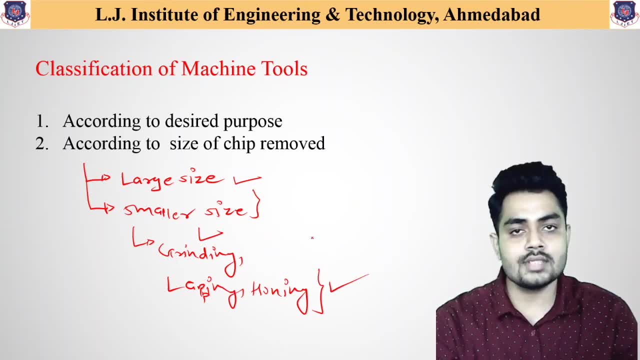 chip during machining operation. so these are called as the small size chip removed and normal machineries, that is, the maybe a lathe machine milling machine. so these all machineries are nothing but the large size chip removed machineries. so this is the second classification for the machine tools. now 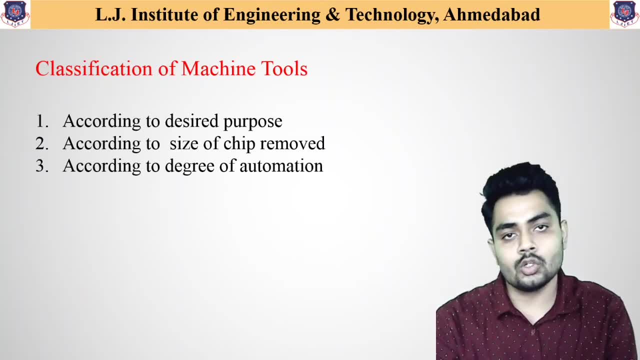 the third one that is according to the degree of automation- so that means it is further classified- is first, one is manual, second one is semi-automatic and the third one is fully automatic machine tools. so first, in manual machinery, if we say all the operation needs to be fully automated, we need to have the meaning manual company type goes there. 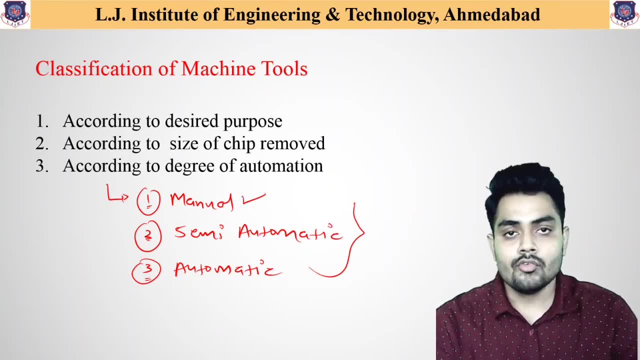 performed by particular labor only, whereas in the semi-automatic machine tools some of the movement to the tool is provided by using the motor or any other further a driving mechanism, and some of the application or some of the movements are performed by the labor and the last one, that is, the full or fully. 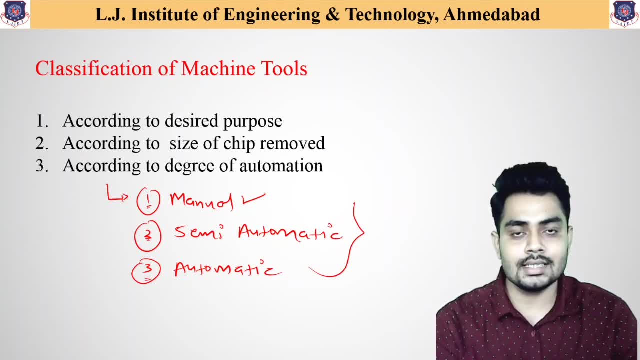 automatic machine tool and in this case, as we have known, the CNC machine tool. that is the fully automatic, in which all the operation, from converting raw material to the final finished product, it is fully converted into that CNC machine. so there is no any labor work required. so that's why it is called as 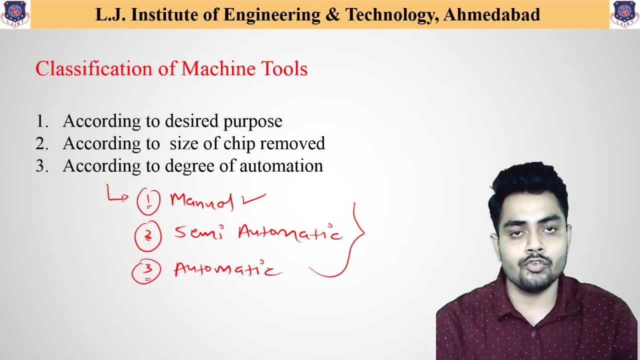 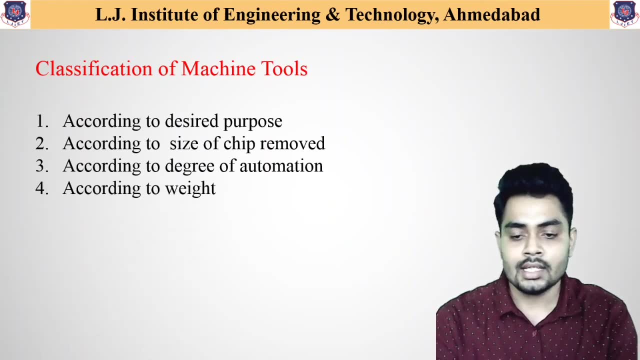 the automatic degree or automatic machine tool for machining purpose. so, based on this, there are three different variations are available. now let us have a look at fourth one, that is, the according to the weight. so, according to weight, there are different variations of machine tools are also available. that 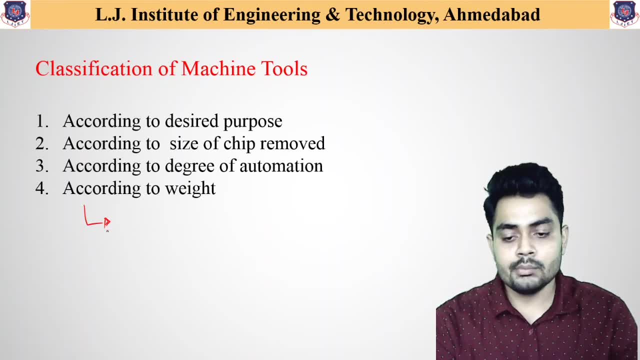 means if the A machine tool is available which has the weight less than 1 ton, then it is one category. if the machine tool has weight in the range of 1 ton to 10, at that time it is in the range of 1 to 10 and machine tool might have a weight greater. 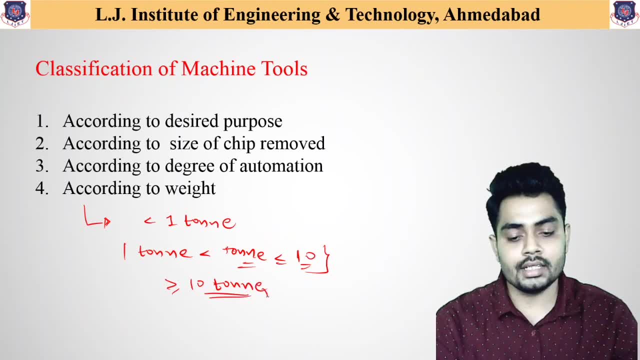 than or equal to 10 tons. so in this case there are three different variations are available. so, based on that, may be a light duty machine tool, medium duty machine tool or heavy duty machine tool. that is how these machine tools can be defined as according to the weight. so these are the four different. 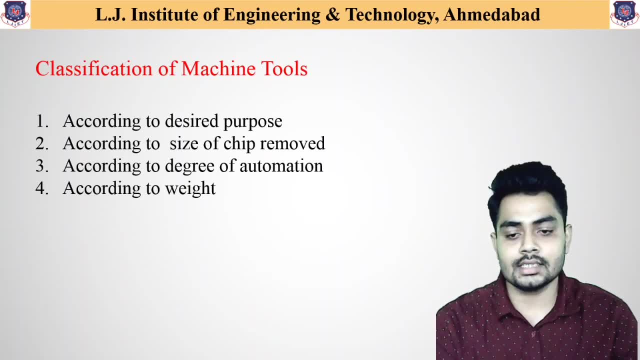 variations are available according to the machine tool classification. so first one, let us further summarize according to the desired purpose, according to the size of chip removed, according to the degree of automation and the last one, that is, according to the weight. so these are main. four major variations are available in the machine tools. now, in any of the machine. 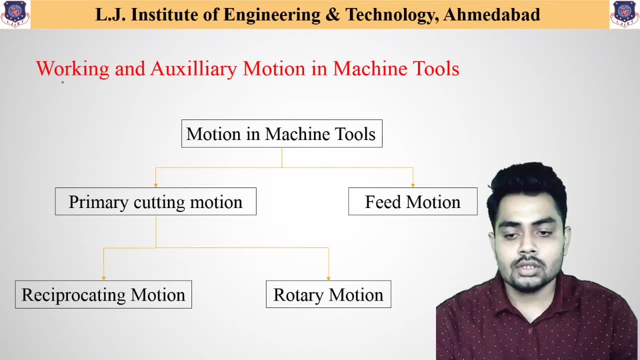 tools to understand that, as we have no first one, that is the working, and the second one, that is the auxiliary motions are available in the machine tools. in our first introductory lecture we have taken the example of the Apple in Apple. if we want to cut that particular Apple, that knife needs to be moved in forward. 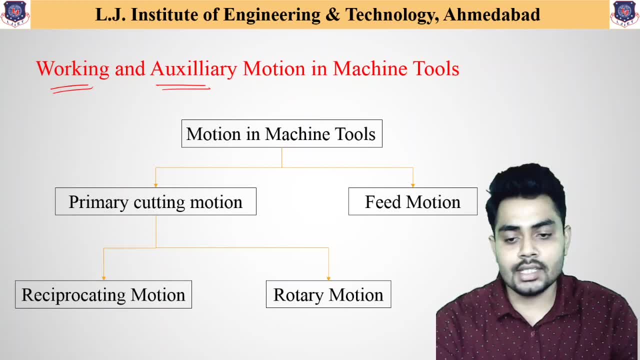 and backward direction for that cutting purpose. so, for that cutting, if we take an example, if we want to cut this Apple, then two moments are required. first one, that is the forward and backward movement of this particular knife, and to cut it up to the end, the another movement required, that is the downward movement. so there, 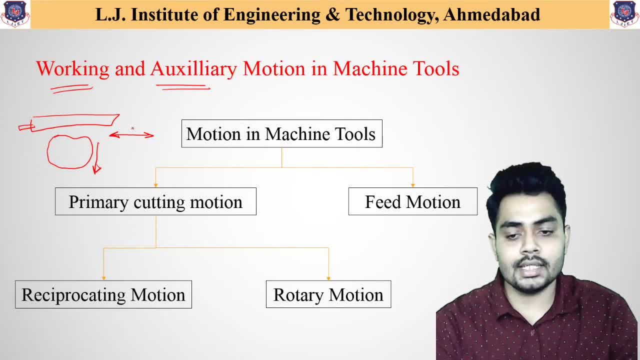 are two moments are requirement, for, from which the first one, that is the forward and backward movement, that is the primary motion, that is the working motion, without which cutting is not possible, and the second auxiliary movement, that is the downward movement, with which entire component or entire Apple can be cut very easily. so that is. 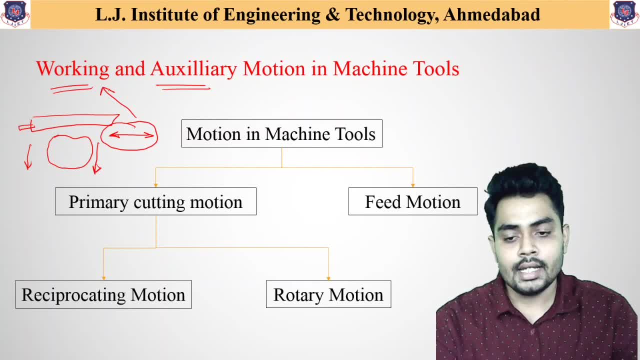 how this first movement is called as the working movement and the bottom movement, or the downward moment, it is called as the auxiliary motion in this simple example. so similarly, in all these different types of the machine tools, the there are different variations of machines are available in which 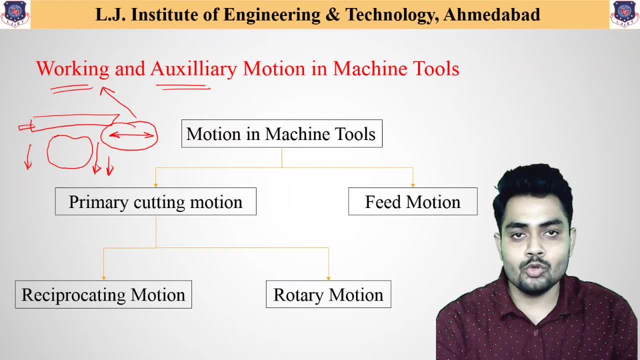 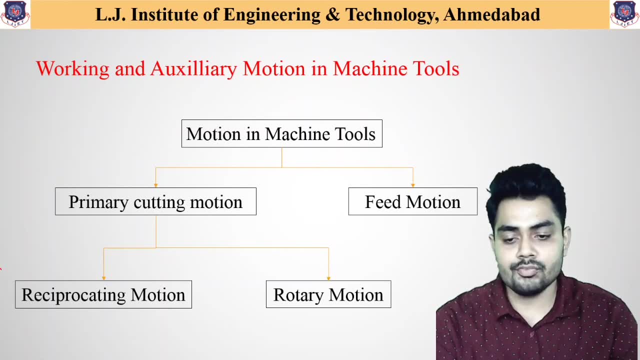 different movements are necessary and these different movements are given by using different mechanisms. so if we summarize further, the motion of machine tool is classified as first one is primary cutting motion and second one, that is the feed motion. and the primary cutting motion is further classified as: first one, that is the reciprocating motion, and the second one, that is the 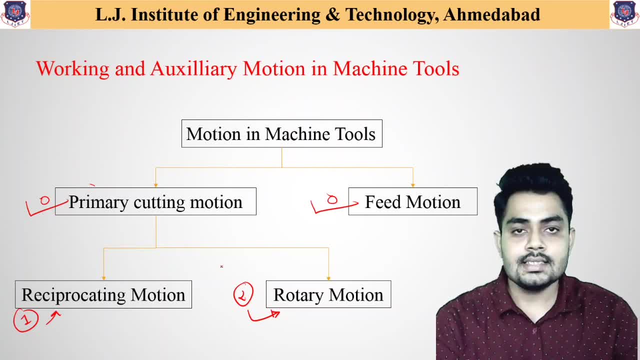 rotary motion. so, as we have discussed in simple case, the first one, that in the case of knife the reciprocating motion is required, there are different machineries are also available in which the rotary movement is necessary, or it is the primary motion to carry out particular operation. so this is there. 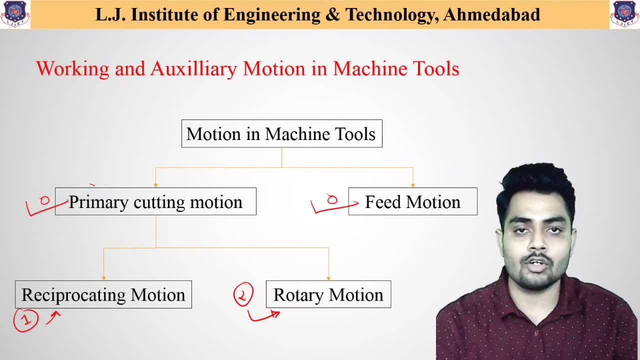 are main, two different variation. first one: the primary motions are of two types. first one is the reciprocating motion and the second one is the rotary motion getting tapped and the second one that is the rotary tap and in second, reciprocating or the main feed motion, that is our auxiliary movement. and these 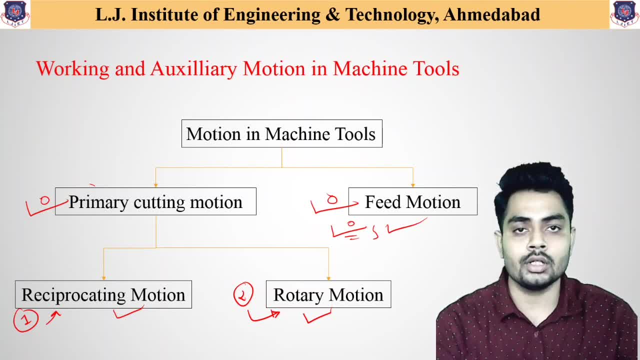 auxiliary movement is required further to cut the component up to certain depth. so these are main, two different variation- it may be a primary or it may be an auxiliary movement- that are considered for machining purposes. so as we have discussed up to now in this lecture, first we have discussed about 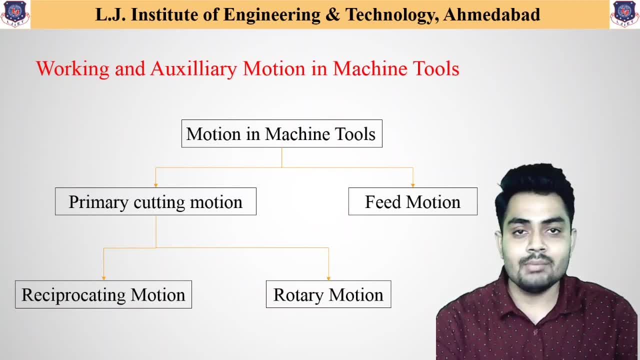 the main major retire, that is, what is the manufacturing, what are the different types of manufacturing processes? then, second, we have discussed about classification of the machine tools. that means how that machine tools are classified, and the third one that are the different motions available in any of the.